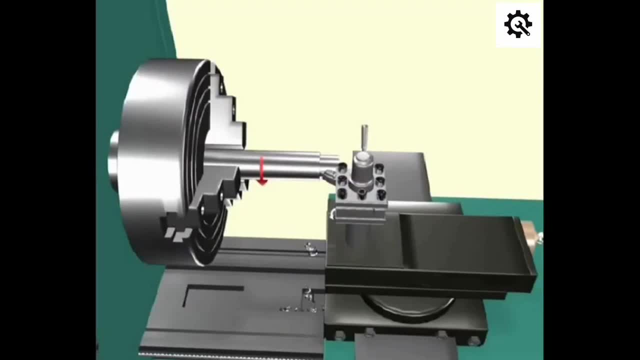 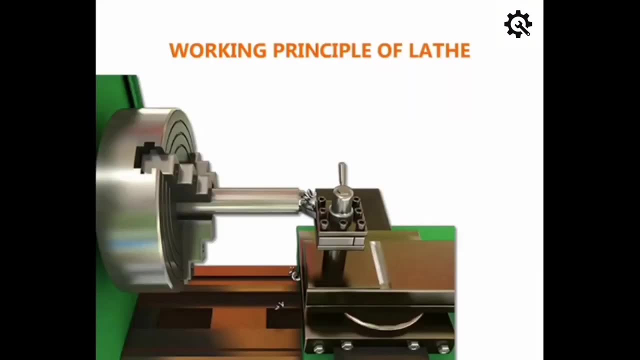 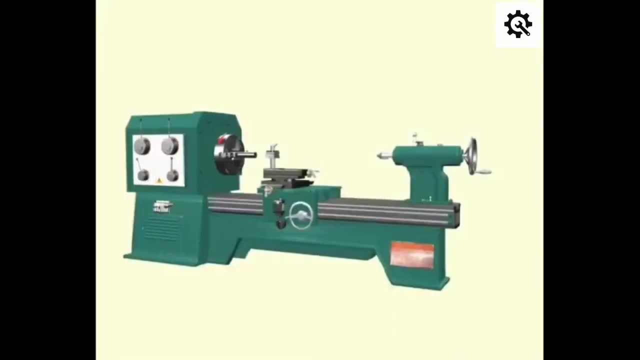 We will discuss about the further details of lathe machine in the next videos. Working Principle of Lathe. In this video we will discuss the working principle of lathe with the help of basic lathe operation. Now we see 3D model of Lathe. 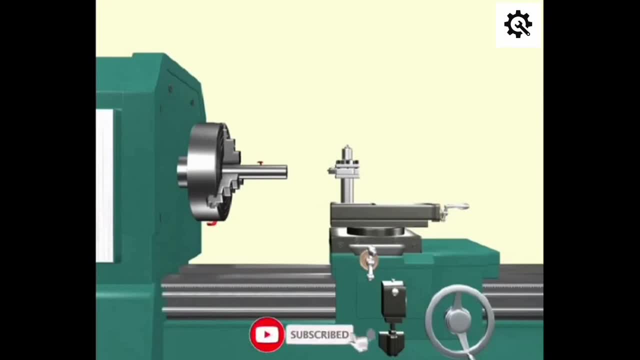 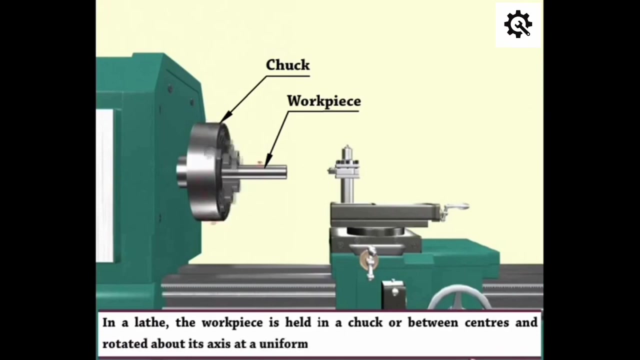 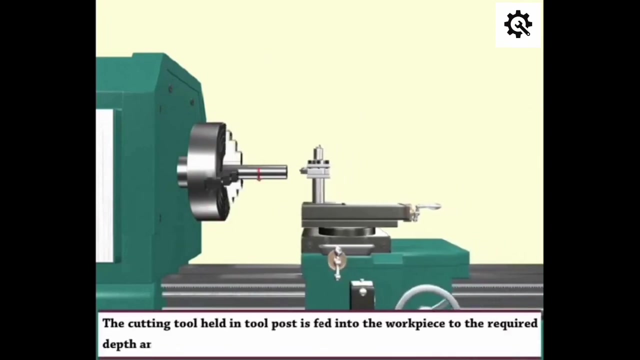 Let us see the principle components of the lathe Workpiece: Lathe- Chalk- Tool post- Cutting tool. In a lathe the workpiece is held in a chalk or between centers and rotated about its axis at a uniform speed. The cutting tool held in tool post is fed into. the workpiece. The cutting tool held in tool post is fed into the workpiece. The cutting tool held in tool post is fed into the workpiece. The lathe is rotated to the required depth and in the desired direction. The workpiece is rotated with a cutting tip. 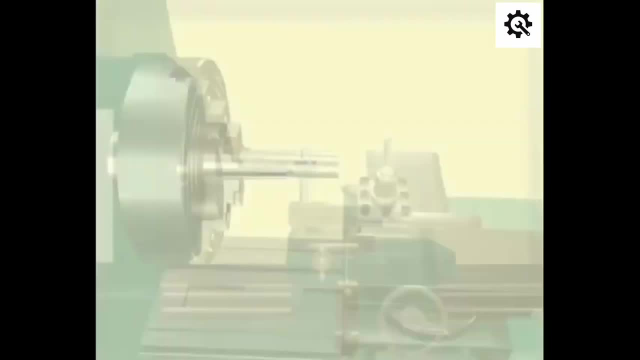 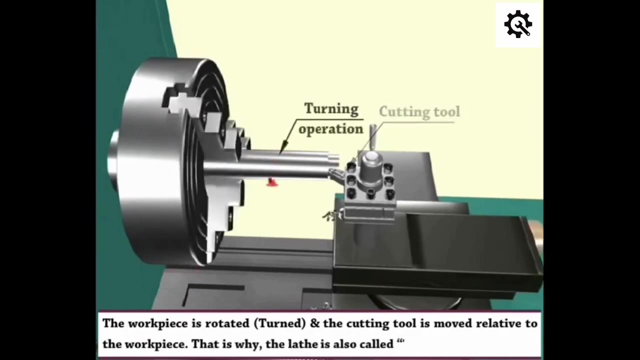 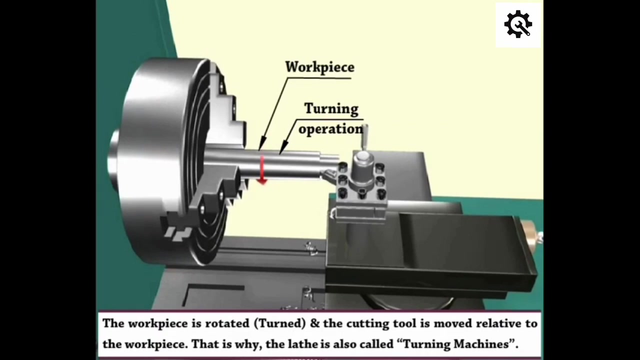 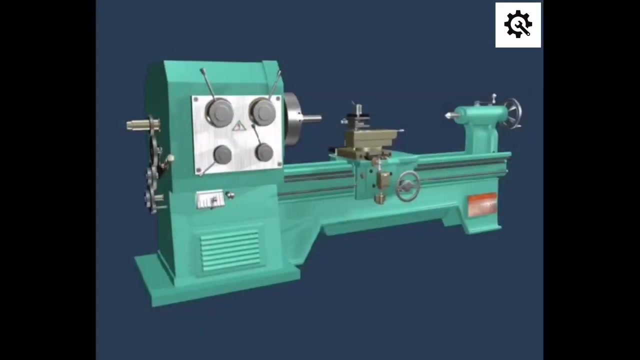 And the cutting tool is moved relative to the workpiece. that is why the lathe is also called as turning machine. CONSTRUCTIONAL FEATURES OF A LATHE. In this video we will discuss about the construction features of center lathe. Firstly, it is nice to know that the lathe, while rotating, is oriented with the center. 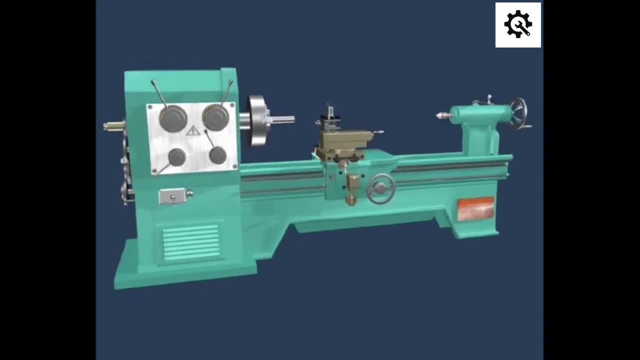 lathe. the middle lathe is considered to be centered. The con为 to radial lathe is a stretch between the80 degrees and the talking lathe may make it difficult to feel when the lathe rotates with the center first. Headstock assembly. 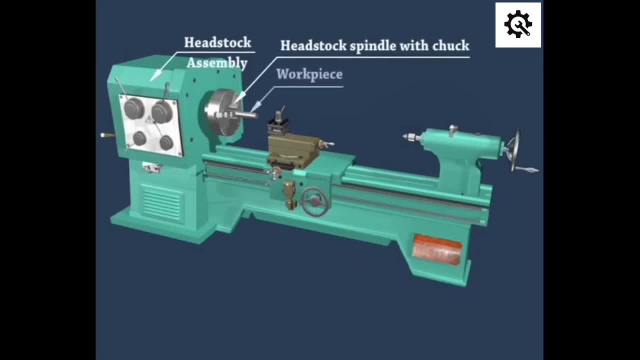 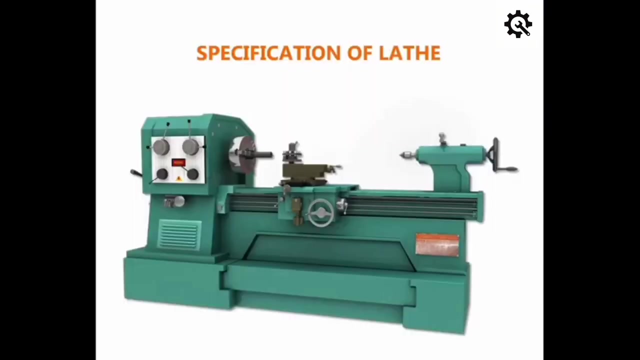 Headstock, spindle with chuck, Workpiece, Tweed, selector. Tailstock assembly- Dead center Carriage assembly, Compound, rest Apron, Cross slide Tool, post Lathe, bed Guide ways, Lead screw, Feed rod. Specification of lathe. In this video we will discuss about the specification of lathe. 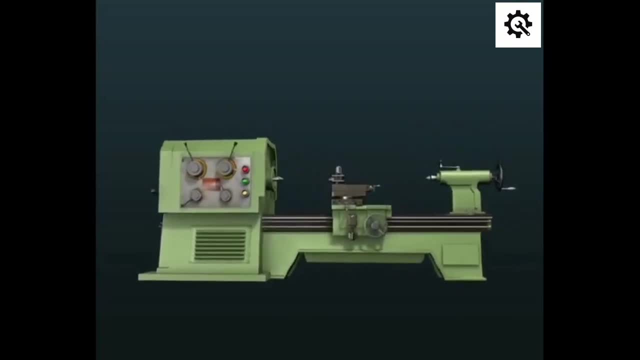 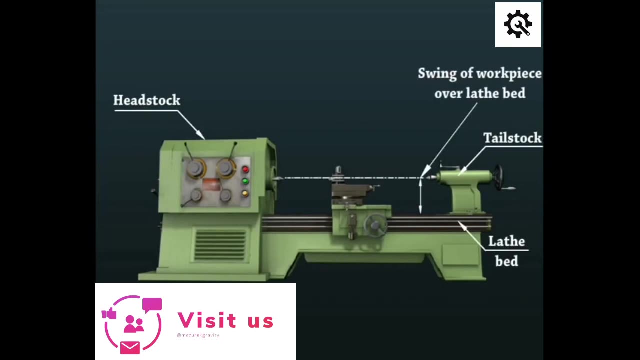 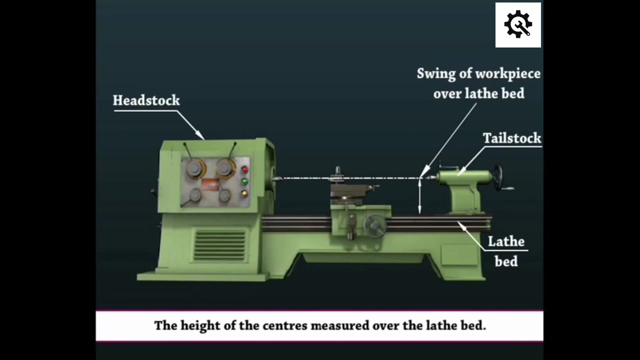 Specification of lathe Descripted in the following ways: Headstock, Tailstock. Lathe bed. Swing of workpiece over lathe bed. The height Length of the center measured over the lathe bed. Swing over the carriage Swing or diameter over carriage. Distance between centers. Maximum job length in millimeter that may be held between the centers. 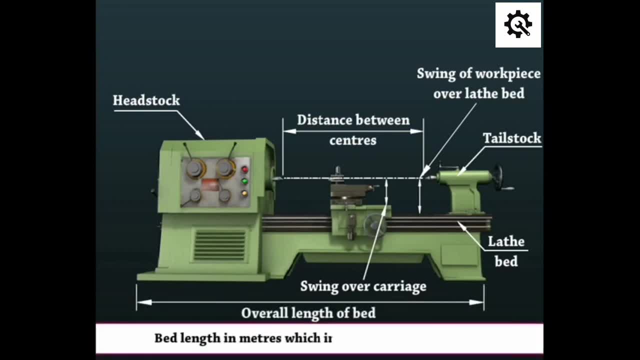 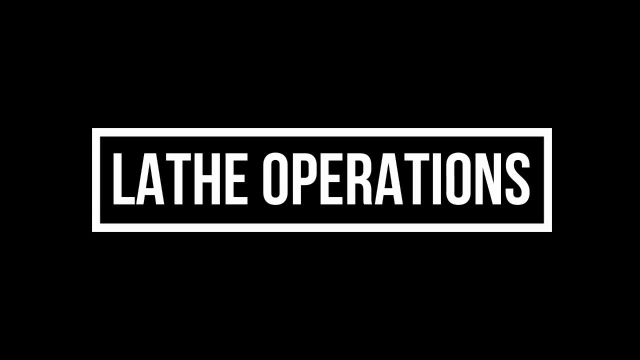 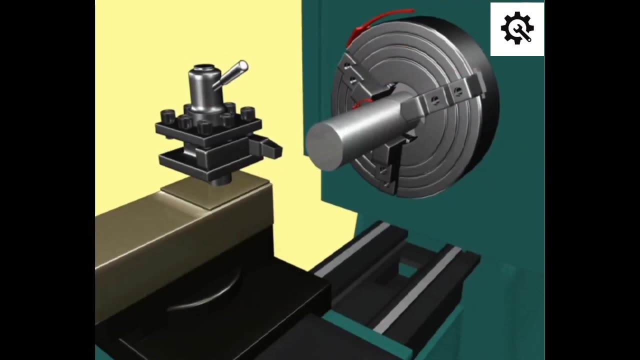 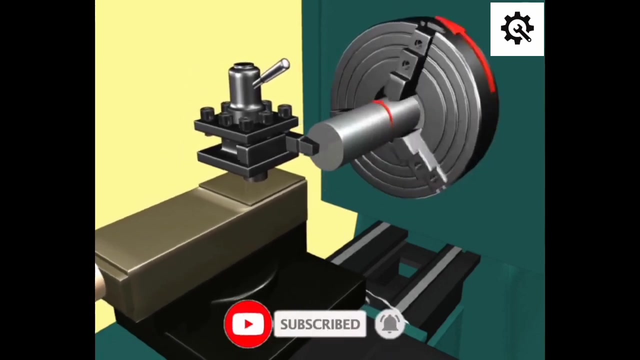 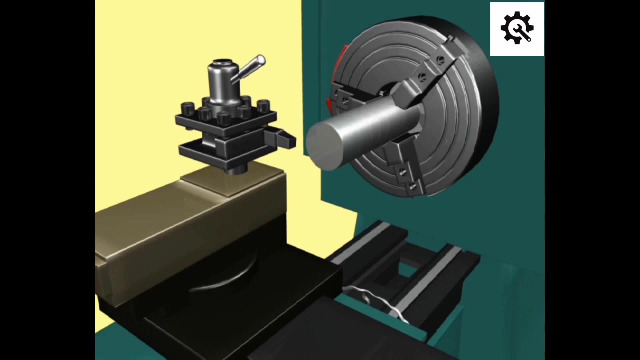 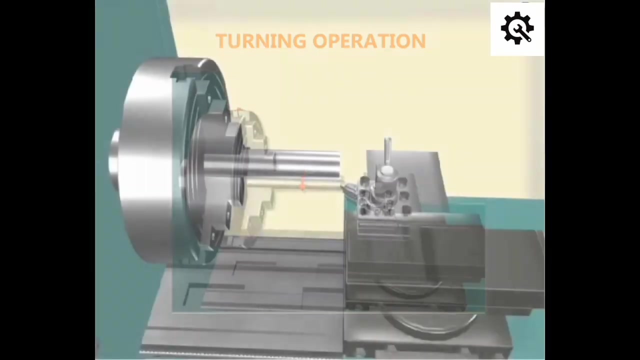 Overall length of bed: Bed length in meters, which includes Headstock length. Let's take a look at the Headstock length. Headstock length is the length of the headstock length is the length of the headstock length when it moves. Thank you for watching.